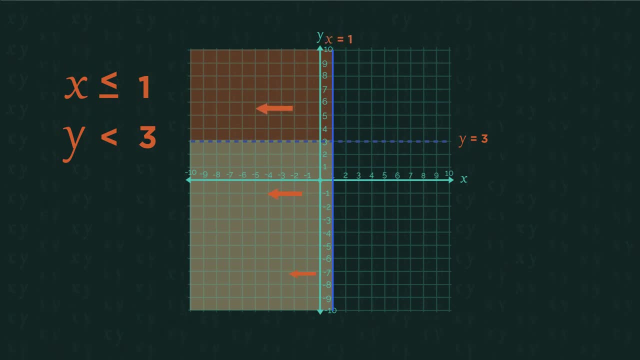 1, because for x we want everything that is less than 1.. And then, looking at y, equals 3.. It's a dotted line, It's a solid line because there's no or equals 2.. And we shade everything underneath the. 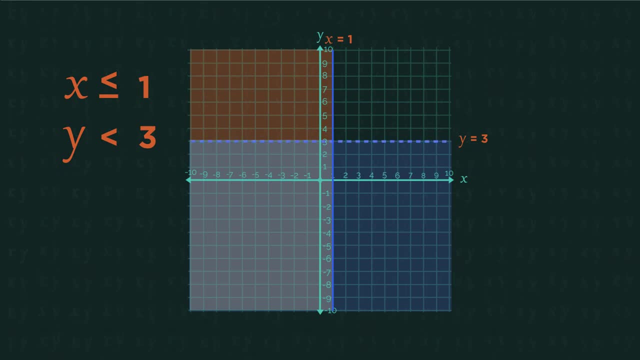 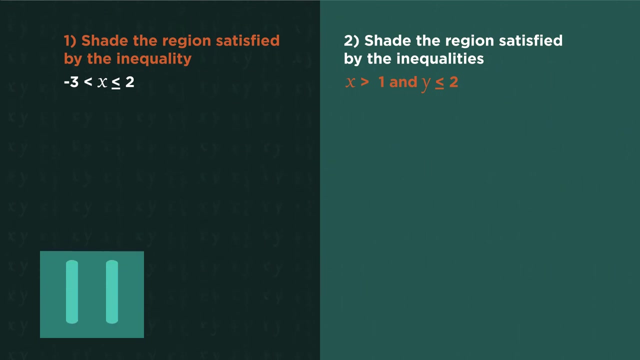 line, because we want everything that's less than 3.. The area that satisfies both inequalities is this section here. So that's the region that we want. Here's two for you to do: Pause the video, shade the region and click play when you're. 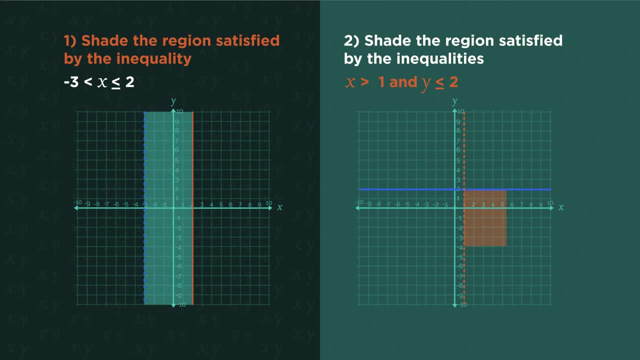 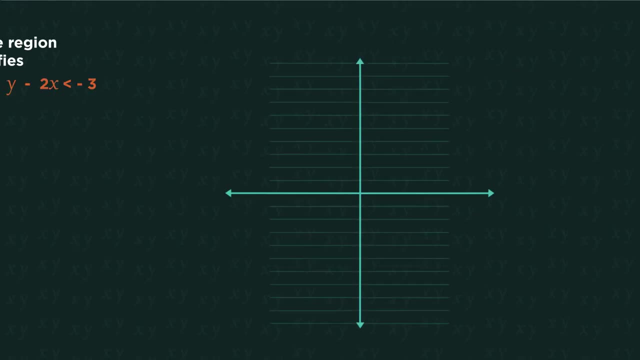 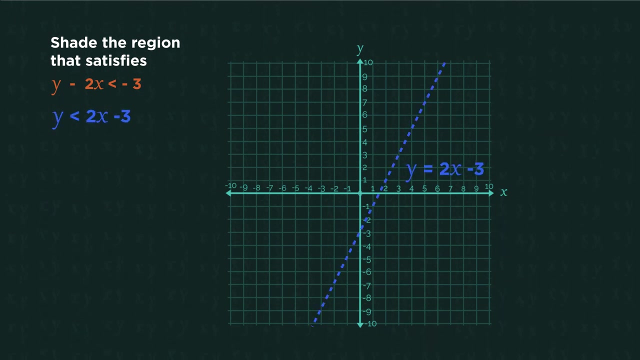 ready? How did you get on? What if we have diagonal lines? We first need to rearrange the equation to make y the subject, Then plot this line onto the graph with a dotted line. because there's no or equals 2. Because the inequality is. 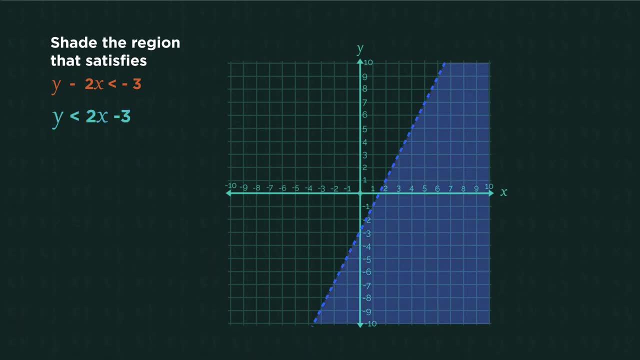 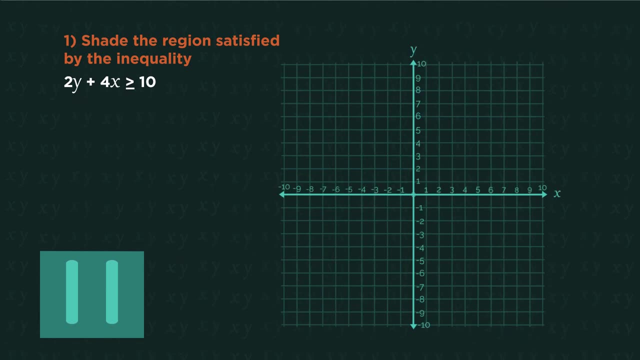 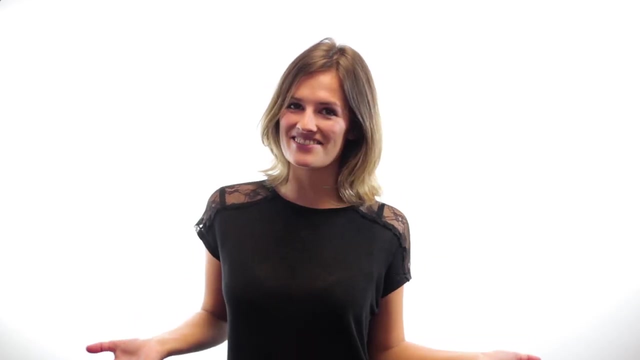 less than the line. we shade everything underneath the line. Here's one for you to do: Pause the video, shade the region and click play when you're ready. Did you get it right? We can even shade regions that are bound by multiple inequalities. Start by plotting all. 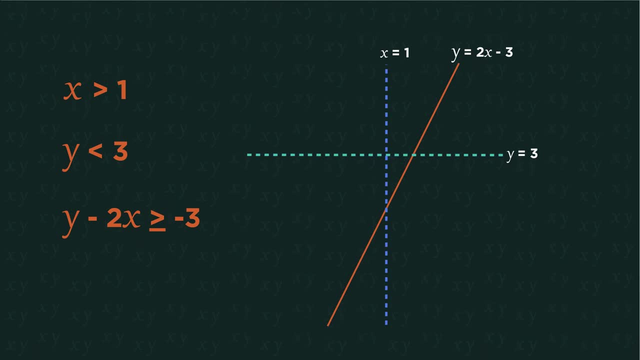 three lines onto the graph, Then do the shading. X is more than 1 is this way, Y is less than 3 is down here, And y is bigger than y is here. So this is our line. Yeah, Isn't that fun. 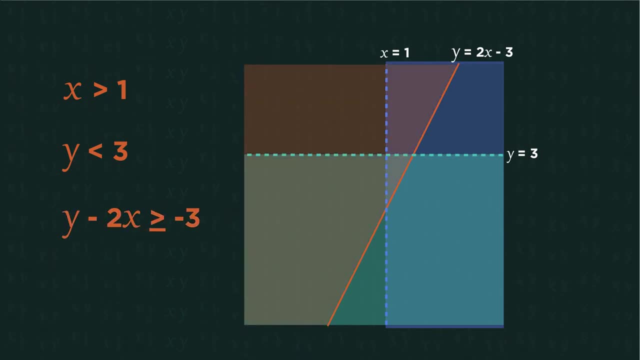 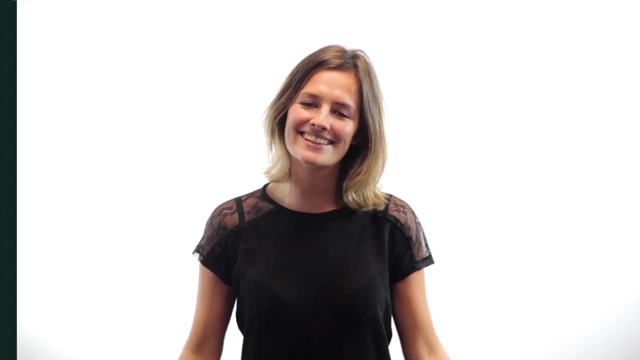 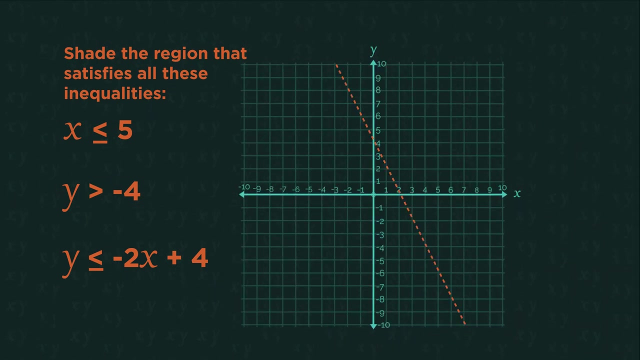 then the line is here: The only region that has been shaded by all three is this bit. So that's the answer. Give this one a go. pause the video, shade the region and click play when you're ready. Did you get it right? So there we have graphing inequalities- The only new thing. 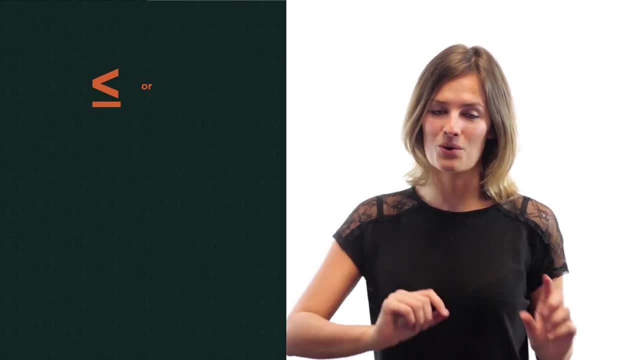 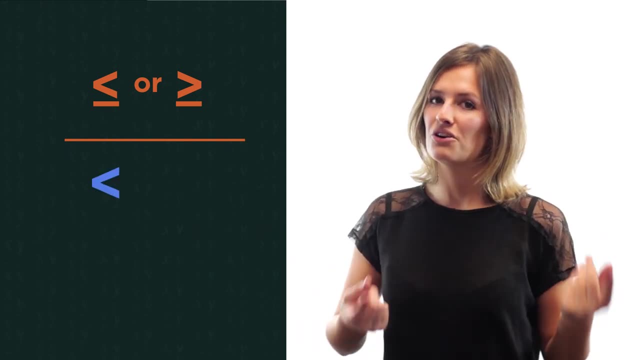 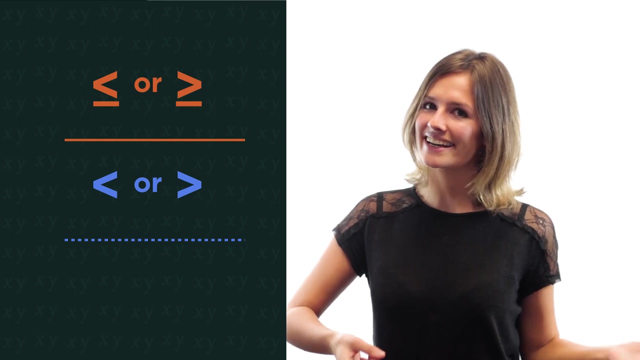 to remember is that if the inequality is or equal to, then it's a solid line. However, if it's just more than or less than so, it's missing. the or equals to part. it's a dotted line. It's missing part of the line. If you liked the video,